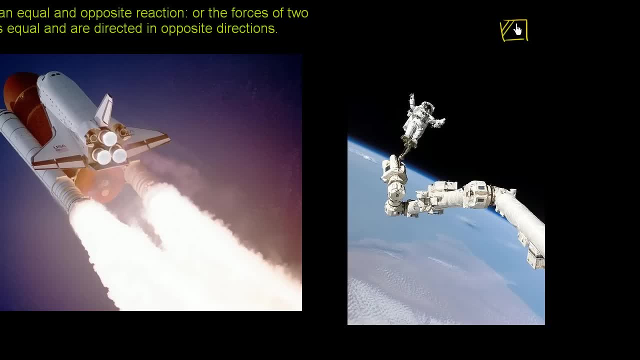 Let's say that I have a some type of block right over here and that I move and I press on the block and I try to push it forward. So this is my hand, this is my hand trying to, trying to press on the block and exert a force, a net force, in that direction so that the block moves to the right. 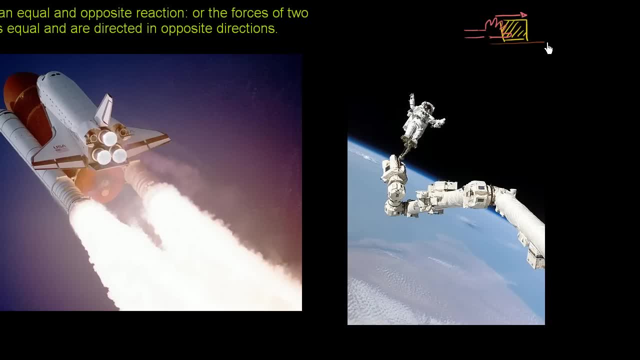 Maybe we, maybe this block is sitting on some type of ice so that it can move. So let's say that I have some. that's a block. Doesn't look like ice. do it in a more ice-like color, So the block is sitting on maybe some ice like that. 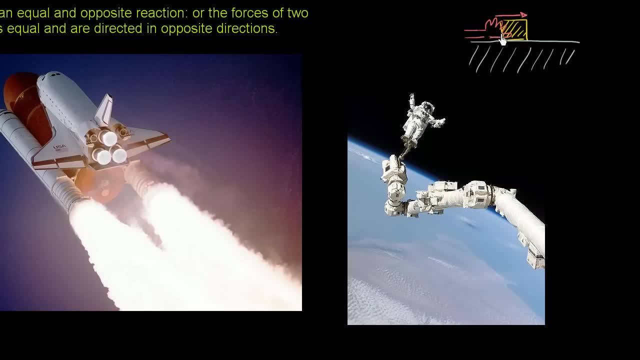 So Newton's third law saying: look, I can press on this block and sure, I'll exert a net force on this block and that net force will accelerate the block, assuming that I can overcome friction, And if it's on ice I can do that. 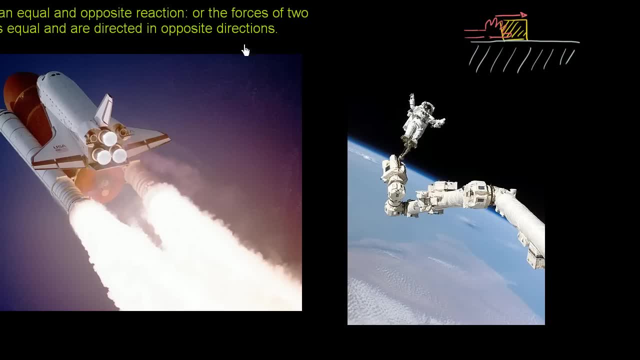 But that block is going to exert an equal and opposite force on me. an equal and opposite force on me And for direct evidence, this is something, Even though it might not be so intuitive when it's said, this equal and opposite force. but direct evidence that it's exerting an equal and opposite force is that my hand will get compressed. 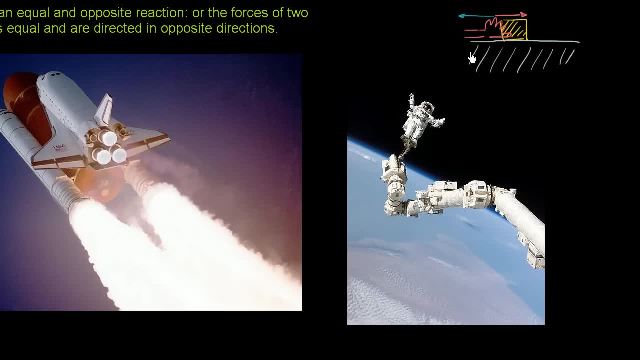 I could actually feel the block exerting pressure on me. Take your hand right now and push it against your desk or whatever you have nearby, and you are clearly exerting a force on the desk. So let me, let me draw. So let's say I have a desk right here. 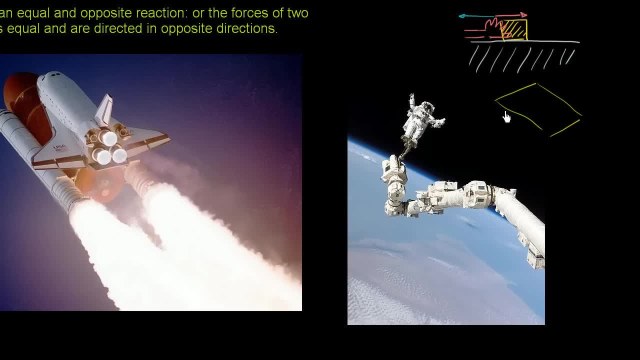 And if I, if I try to push on the desk. So, once again, this is my, these are my, that's my hand right here pushing on the desk. If I push on the desk- and I'm actually doing it right now while I record this video, you'll see so I'm clearly exerting a force on the desk. 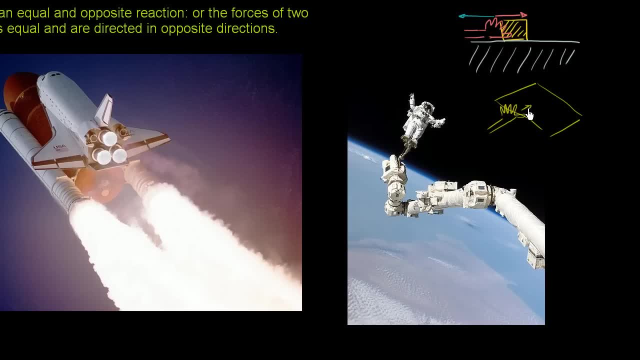 If I do it hard enough, I might even get the desk to shake or tilt a little bit- and I'm actually doing that right now. But at the same time you'll see that your hand is getting compressed. The palm of your hand is being pressed down. 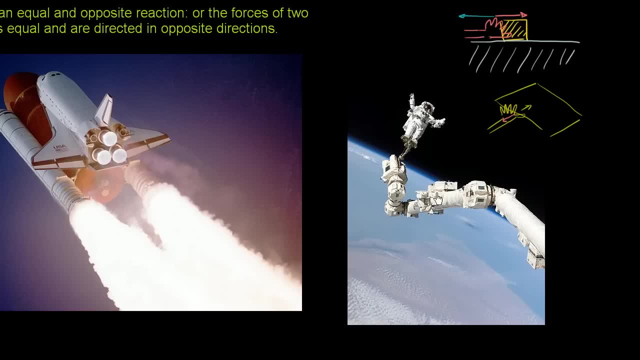 And that's because the desk is exerting an equal and opposite force on you. If it wasn't, You actually wouldn't even feel it, Because you wouldn't even feel the pressure It would feel. your hand would be completely uncompressed. Another example of that: 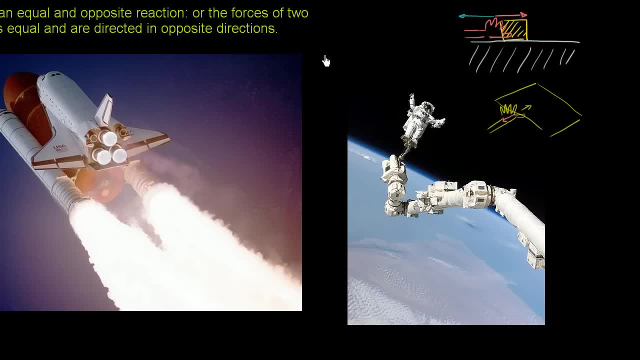 Say you're walking in the beach, Say you're walking on the beach And you have some sand right here. If you were to step on the sand, So let's say that this is your shoe. Do my best attempt to draw a shoe. 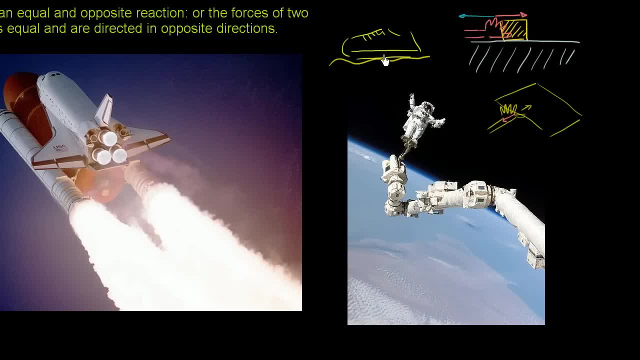 So this is the shoe, If you were to step on the sand, Clearly you are exerting a force on the sand. You are exerting a force on the sand. The force that you're exerting on the sand is the force of your weight. 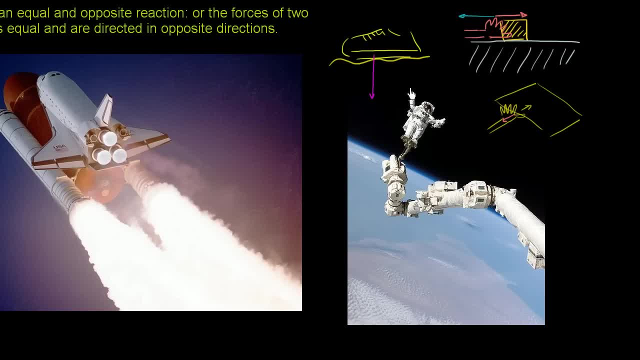 The gravitational attraction between you and the earth. You're exerting that on the sand. The sand is also, and another evidence of that Is that the sand is going to be displaced. You're going to create a footprint. The sand is going to move out of the way. 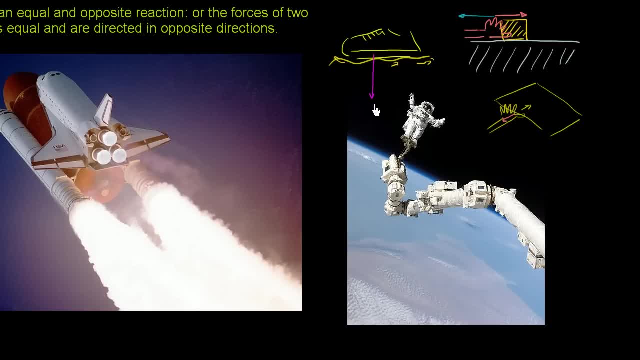 Because it's being pushed down so hard. So clearly you are exerting a force on the sand, But the sand is also exerting an equal and opposite force on you. Is also exerting an equal and opposite force on you, And what's the evidence of that? 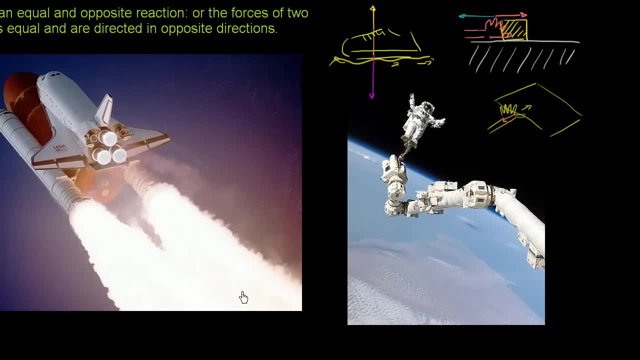 Well, if you believe, If you believe, If you believe Newton's second law, If you have this gravitational force on you, You should be accelerating downwards, Unless there is some other force that balances it out. And the force that balances it out. 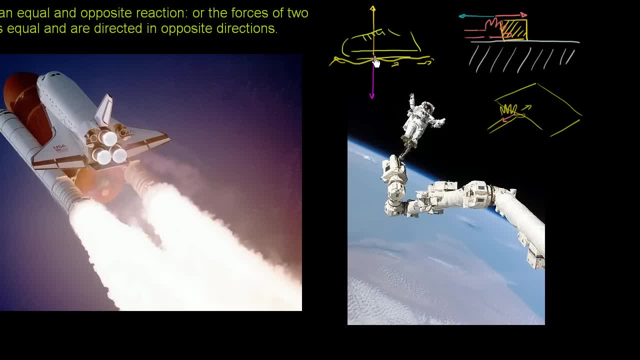 Is the force that the beach or the sand is exerting on you upwards, And so when you net them out, There's a zero net force on you, And that's why you get to stay there, Why you don't start accelerating down towards the center of the earth. 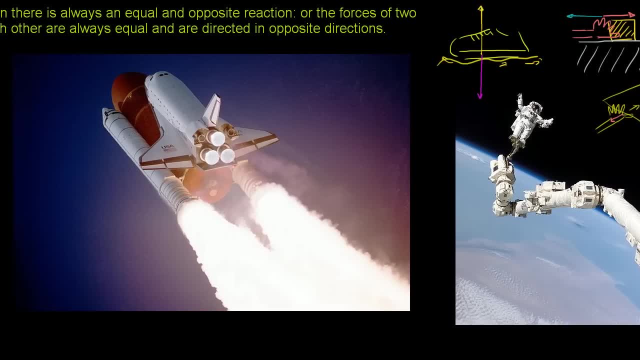 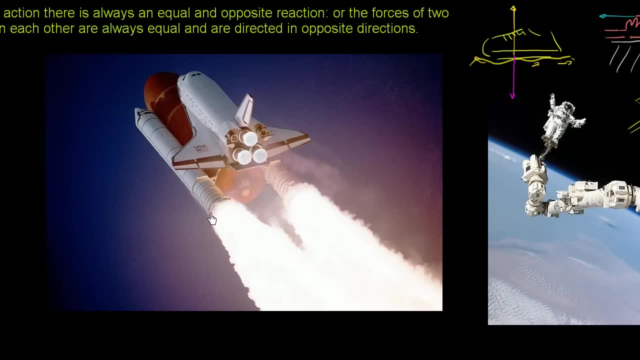 Other examples of this- This is maybe the most famous example of Newton's third law- Is just how rockets work. When you're at a rocket, Either trying to escape the atmosphere Or maybe you're in space, There's nothing to push off of. 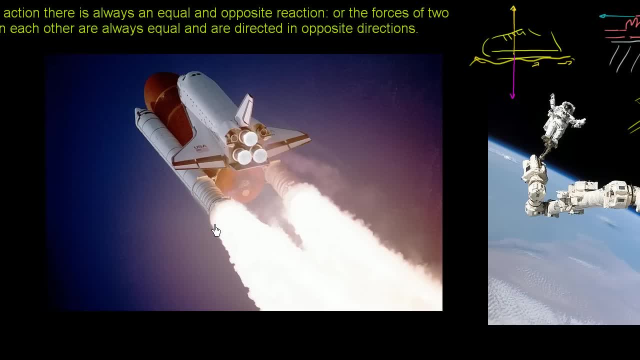 Nothing to push off that let you accelerate. So what you do is You keep stuff to push off in your fuel tanks And when you allow the proper chemical reactions Or the proper combustion to take place, What it does is it expels gases. 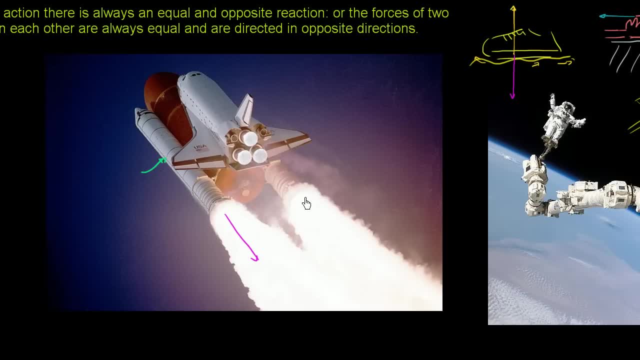 At ultra high velocities Out the back of your rockets. And each of those particles, You're exerting a force on them, Enough force. Even though they're super small mass for each of them, They're going at super high velocity, So they're being accelerated tremendously. 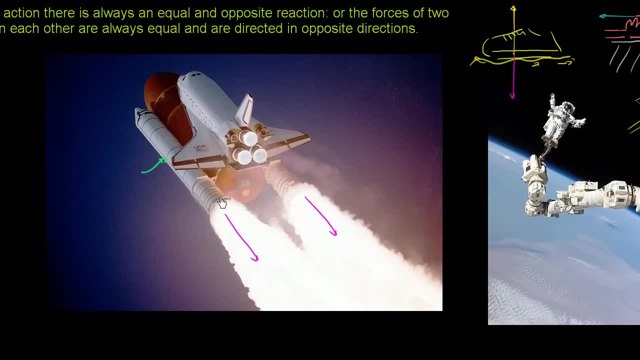 So there's an equal and opposite force on the rocket, The thing that is actually expelling the gas, And so that's what allows a rocket to accelerate, Even when there's nothing In this direct vicinity to push off of. It just expels a bunch of things. 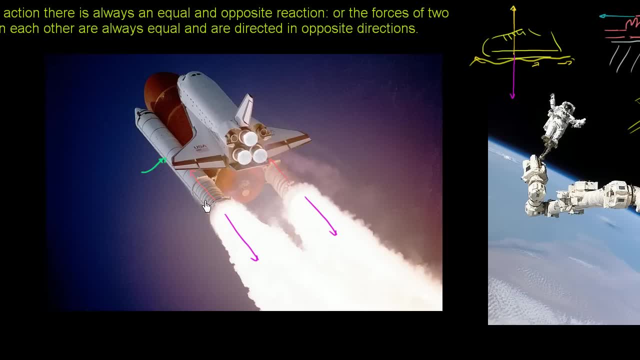 Or it accelerates a bunch of things At a super fast rate, It exerts a force on all these particles And that allows an equal and opposite force To accelerate the rocket ahead. And another example of this Is if you ever find yourself drifting in space. 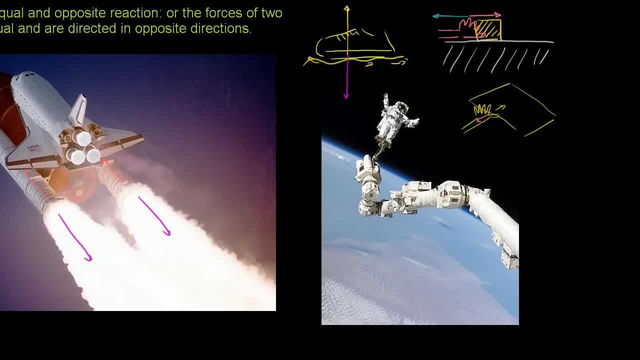 And this is an actual, useful example, So that you don't end up drifting in space forever. Let's say, We don't ever want this to happen. This astronaut: By some chance, He loses his connection To this little tool arm. 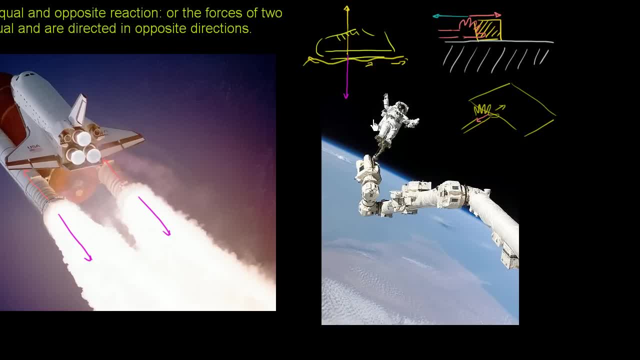 Right here on the space shuttle And he starts drifting away. He starts drifting away. What can that astronaut do To change the direction of his motion So that he drifts back to the space shuttle? Well, you look around. You're like wow. 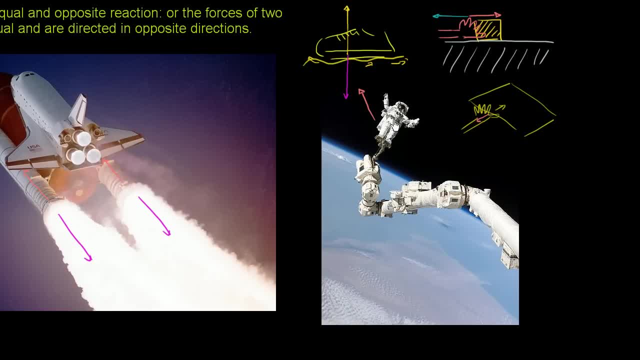 There's nothing to push off of. He doesn't have any wall to push off of, And let's just assume He doesn't have any rocket jets Or anything like that. What could he do? Well, the one thing you could do. 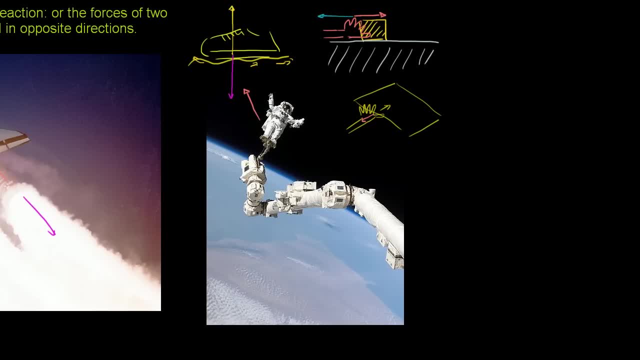 And this is the situation If you're ever drifting in space- Is you should find the heaviest, Or I should say the most massive thing on you, And we'll explain the difference between Between mass and weight in a future video. But you should find the most massive thing. 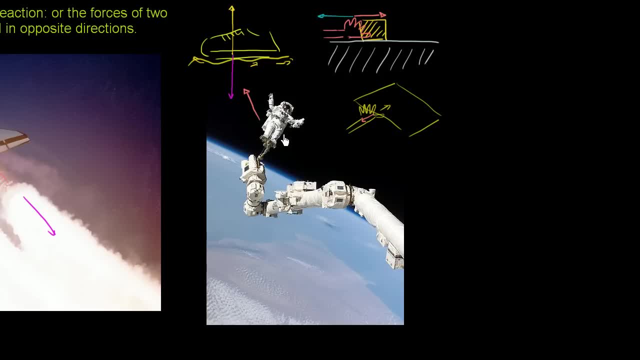 That you can carry, That you can take off of you, That you can throw, And you should throw it in a direction opposite yourself. So let me put it this way: If I throw, Let's say I'm in space And I'm floating. 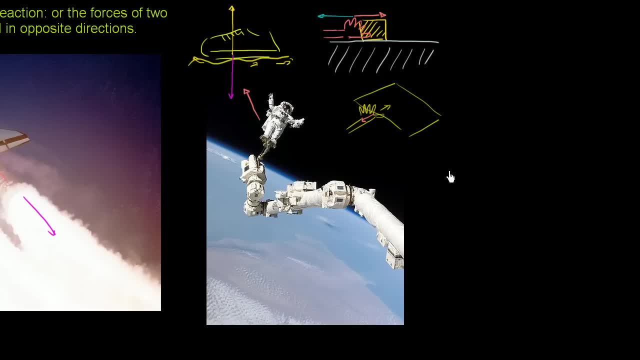 I'll just show it. I'll make it look like the glove of a. So Let's say that this is, This is the glove of the astronaut. There you go. That's his hand. That's the astronaut's hand Right over here.